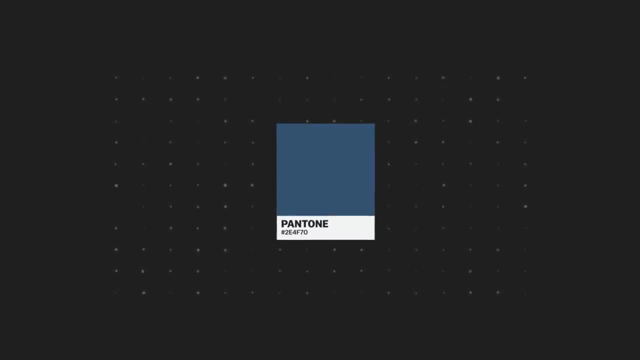 If I showed you this paint chip and asked you to tell me what color it is, what would you say? How about this one And this one? You probably said blue, purple and brown. But if your native language is Wobe from Côte d'Ivoire? 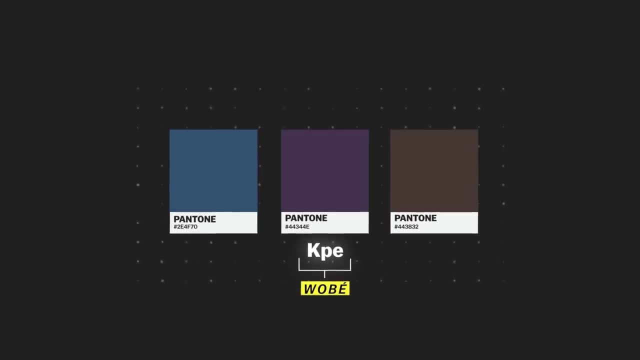 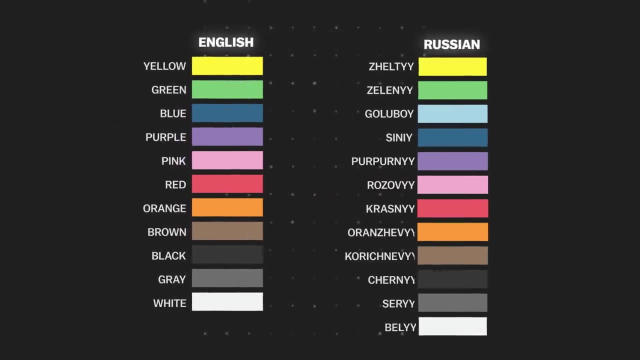 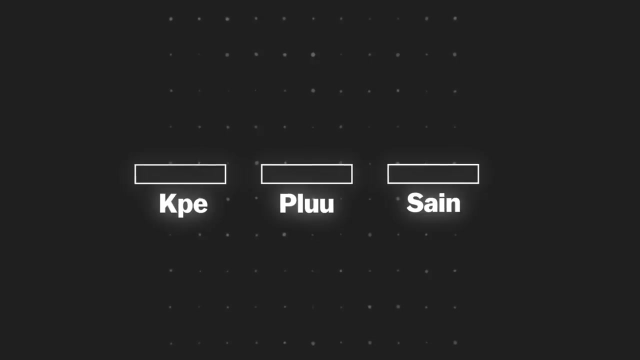 you probably would have used one word for all three. That's because not all languages have the same number of basic color categories. In English we have 11,, Russian has 12, but some languages, like Wobe, only have three, And researchers have found that if a language only has three or four basic colors, they can 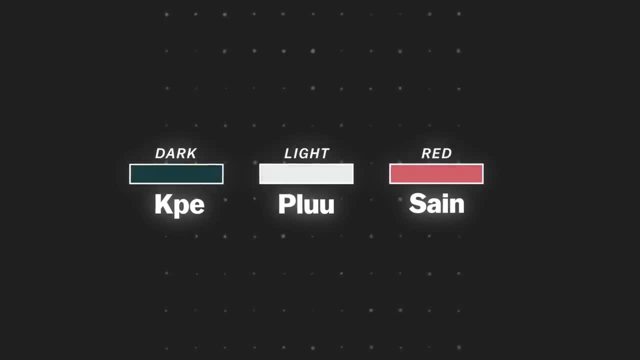 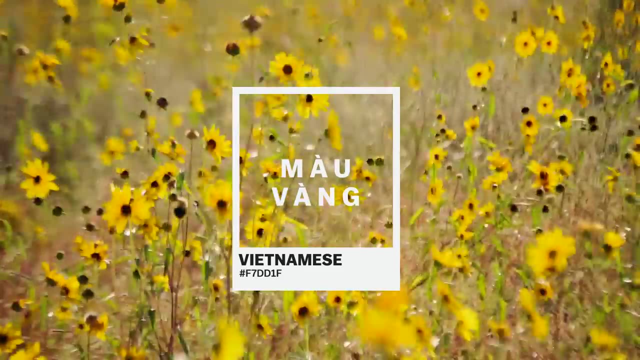 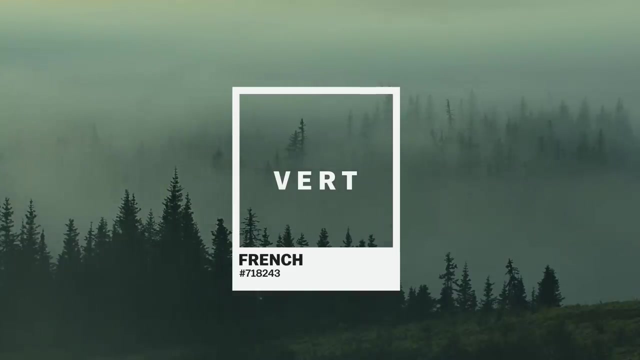 usually predict what those will be. So how do they do it? As you would expect, different languages have different words for colors, But what interests researchers isn't those simple translations. It's the question of which colors get names at all, Because as much as we think of colors in categories, the 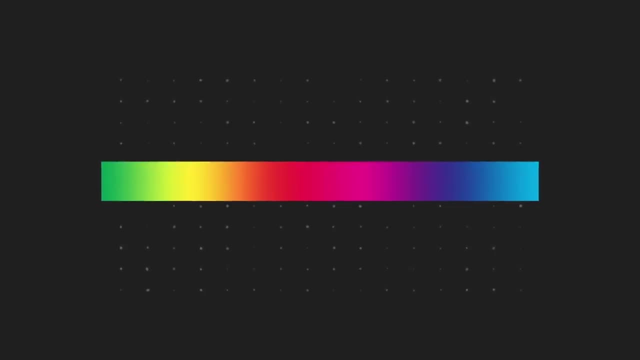 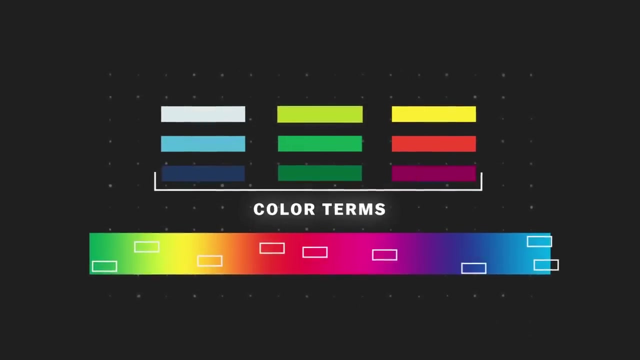 truth is that color is a spectrum. It's not obvious why we should have a basic color term. For example, we can choose a color for this color, but not this one, And until the 1960s it was widely believed by anthropologists that cultures would just. 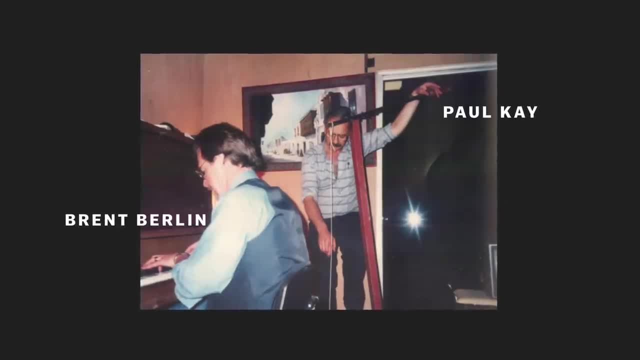 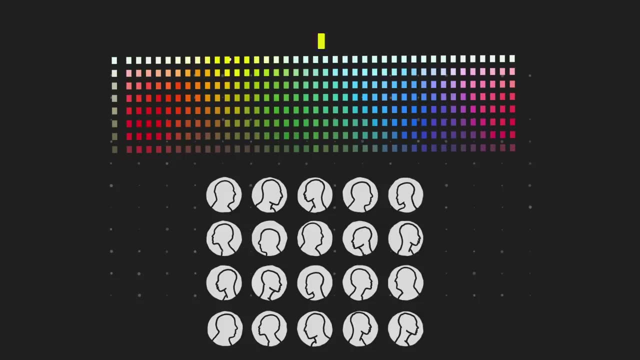 choose from the spectrum randomly. But in 1969, two Berkeley researchers, Paul Kay and Brett Berlin, published a book challenging that assumption. They had asked 20 people who spoke different languages to look at these 330 color chips and categorize each of them by their basic color term, And they found. 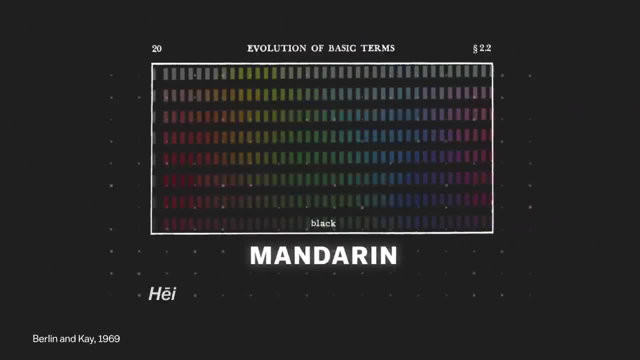 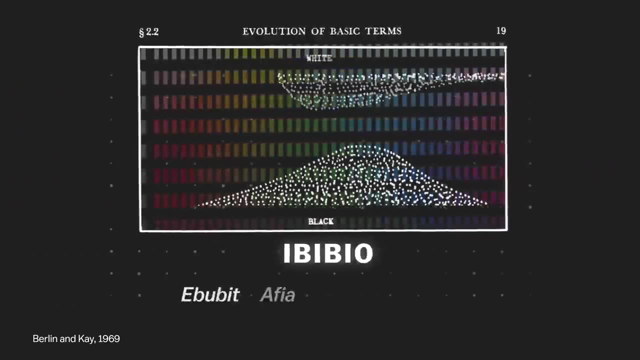 hints of a universal pattern. If a language had six basic color words, they were always for black or dark, red, green, yellow and blue. If it had four terms, they were for black, white, red and then either green or yellow. If it had only three, they were always for. 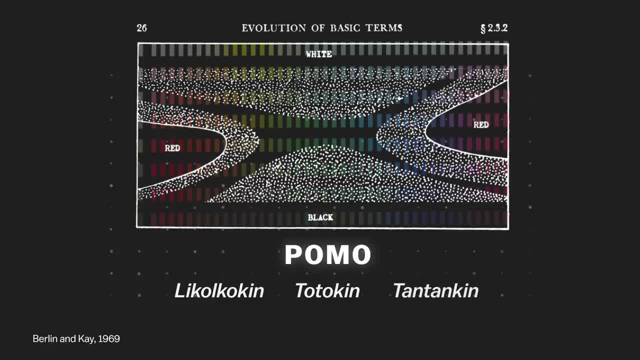 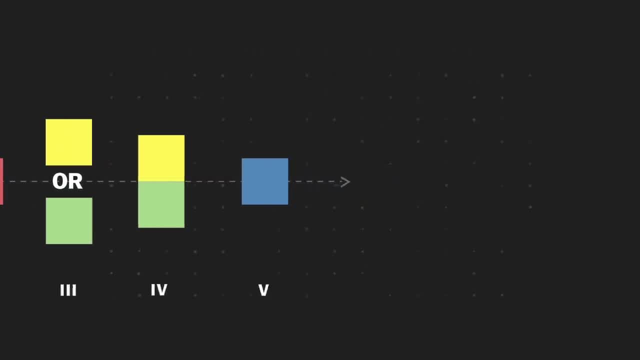 black, white and red. It suggested that as languages develop, they create color names in a certain order: First black and white, then red, then green and yellow, then blue, then others like brown, purple, pink, orange and gray. The theory was: 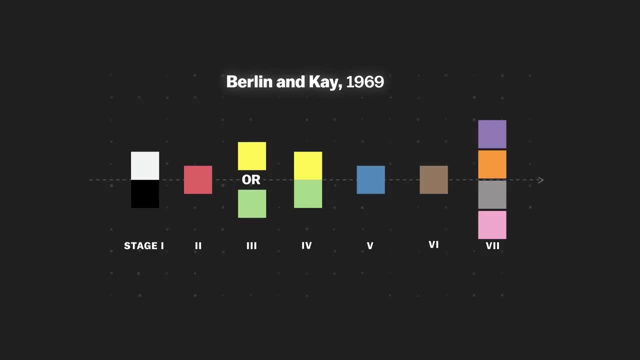 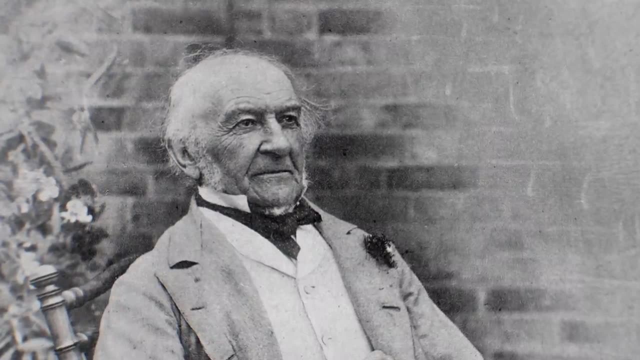 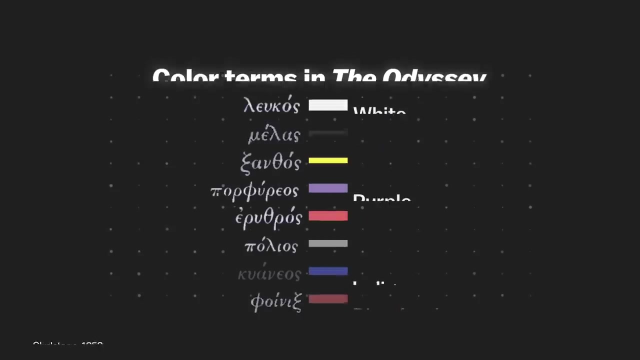 revolutionary. They weren't the first researchers interested in the question of how we name colors. In 1858, William Gladstone, who would later become a four-term British prime minister, published a book on the ancient Greek works of Homer. He was struck by the 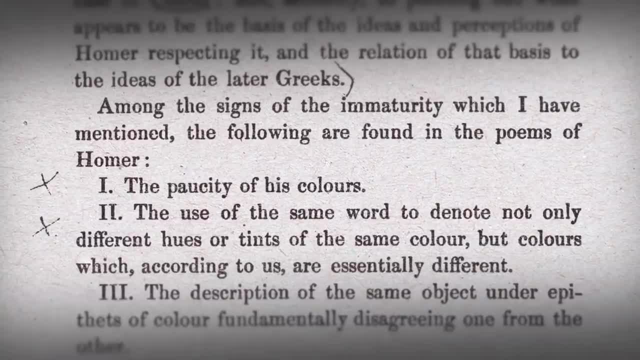 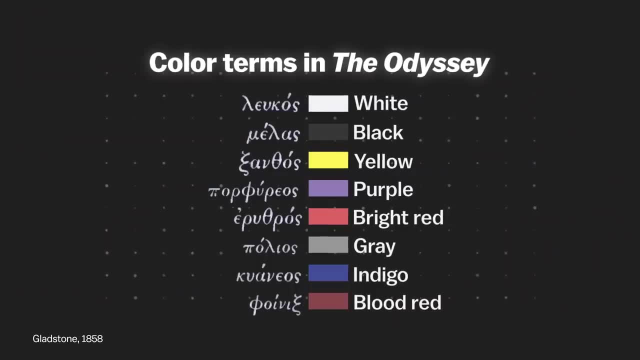 fact that there weren't many colors at all in the text and when there were, Homer would use the same word for quote colors which, according to us, are essentially different. He used the same word for purple to describe blood, a dark cloud, a wave and a rainbow, and he referred to the sea. 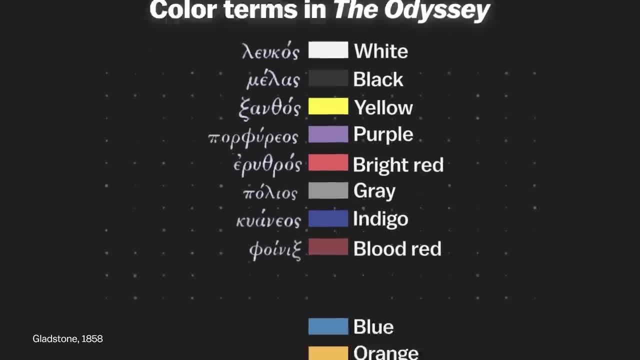 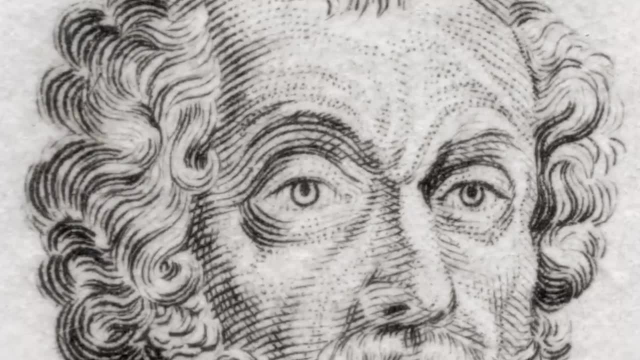 the sea as a white and the sea as a blue and the sea as a white. Gladstone didn't find any references to blue or orange at all. Some researchers took this and other ancient writings to wrongly speculate that earlier societies were colorblind. Later, in the 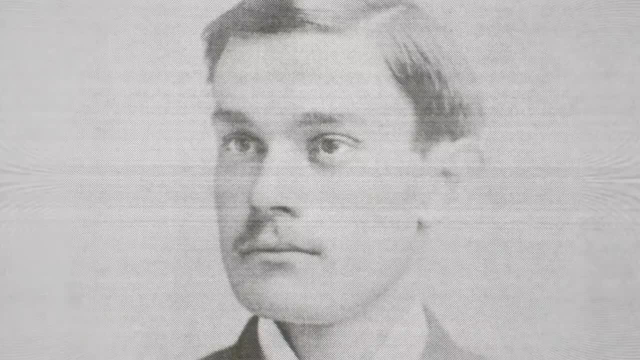 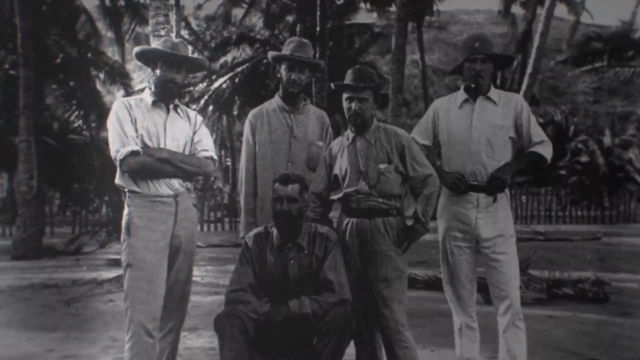 19th century, an anthropologist named WHR Rivers went on an expedition to Papua New Guinea, where he found that some tribes only had words for red, white and black, while others had additional words for blue and green. An expedition to investigate the cultures. 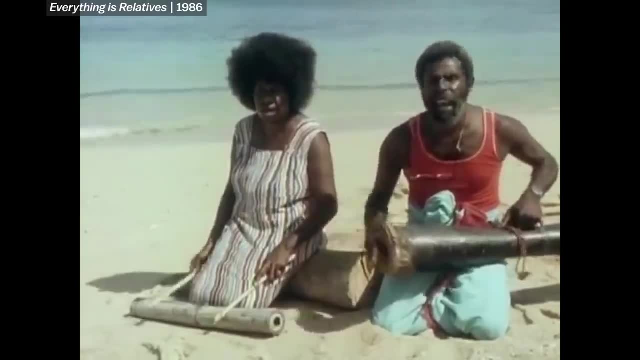 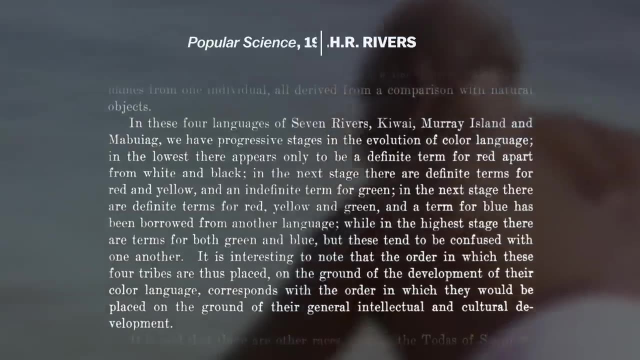 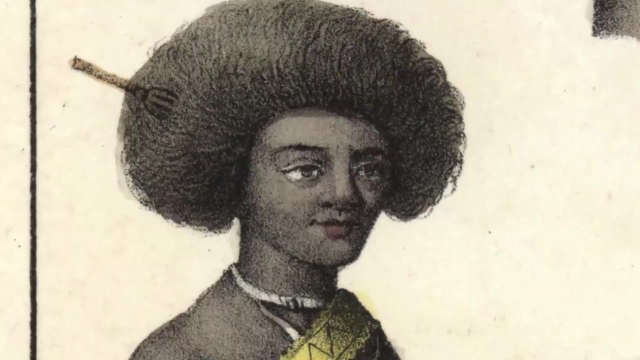 on a remote group of islands in the Torres Straits between Australia and New Guinea. His brief was to investigate the mental characteristics of the islanders. He claimed that the number of color terms in a population was related to their quote, intellectual and cultural development, and he used his findings to claim that 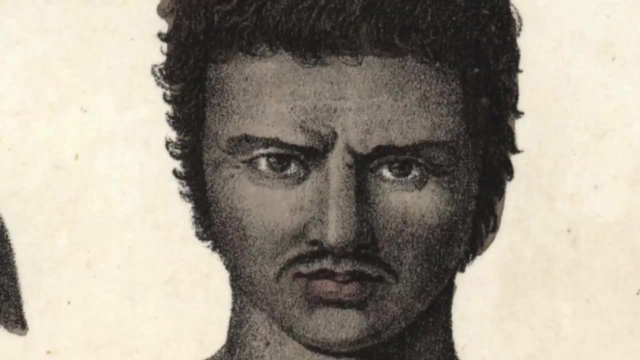 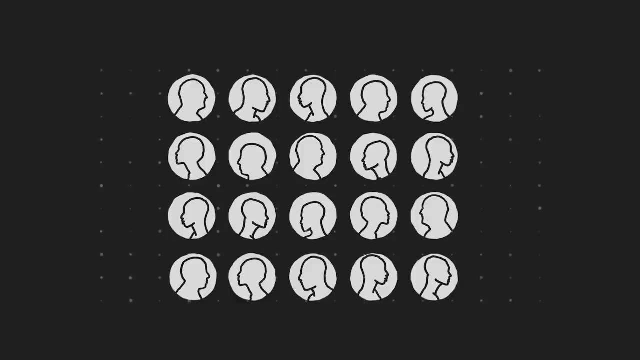 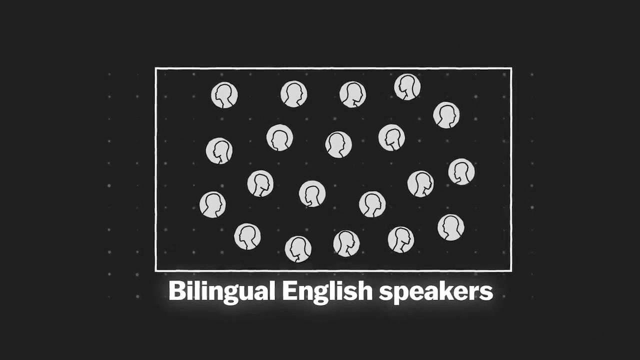 Papuans were less physically evolved than Europeans. Berlin and Kay didn't make those racist claims, but their color hierarchy attracted a lot of criticism. For one thing, critics pointed out that the study used a small sample size- 20 people, all of whom were bilingual English speakers, not monolingual native speakers. And 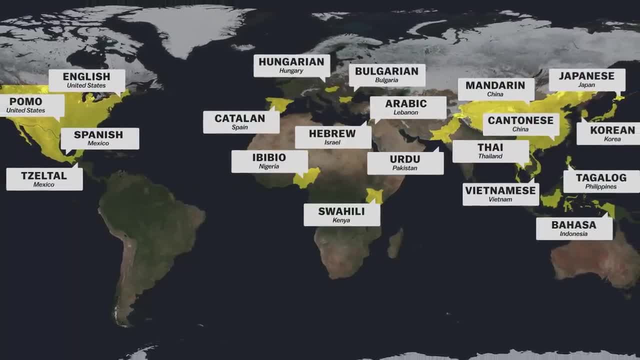 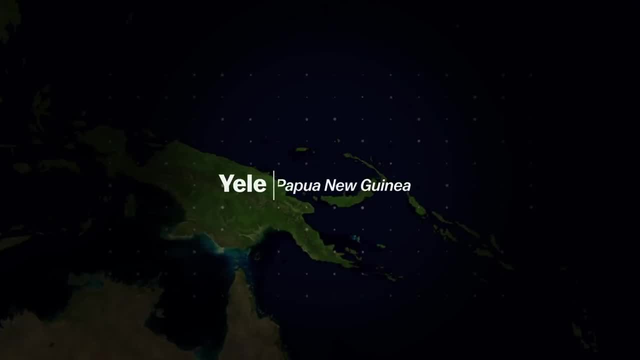 almost all of the languages were from industrialized societies- hardly the best portrait of the entire world. But it also had to do with defining what a basic color term is In the Yelay language in Papua New Guinea, for example. there are only basic color terms for 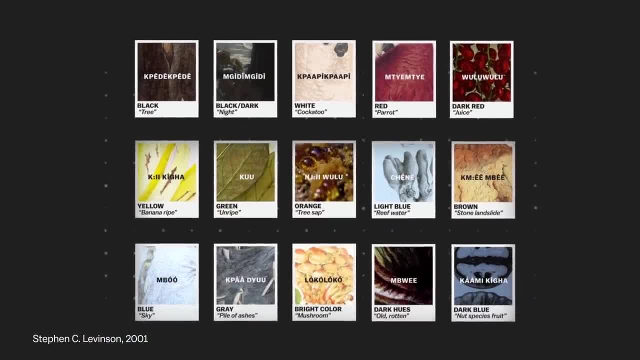 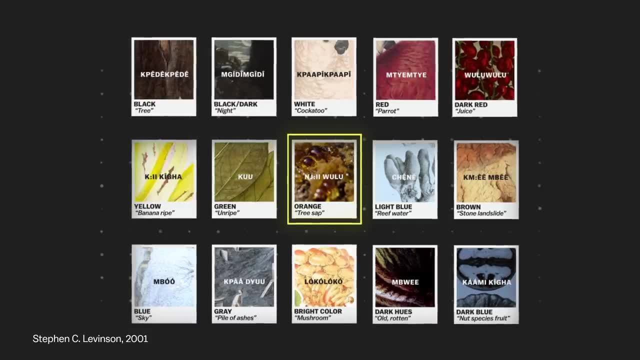 black, white and red, But there's a broad vocabulary of everyday objects like the sky and tree sap that are used as color comparisons that cover almost all English color words. There are also languages like Hanuno'o, from the Philippines, where a word can communicate both. 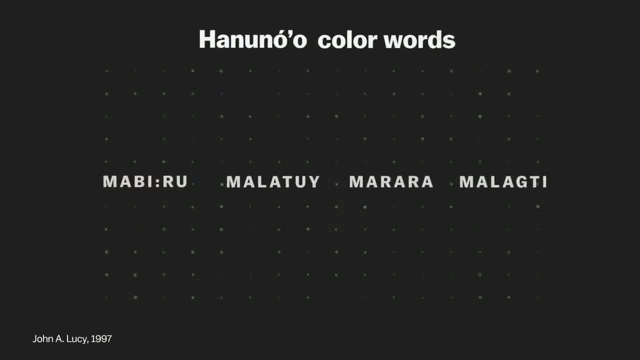 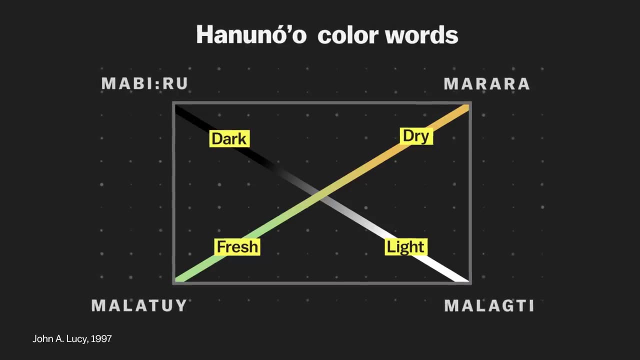 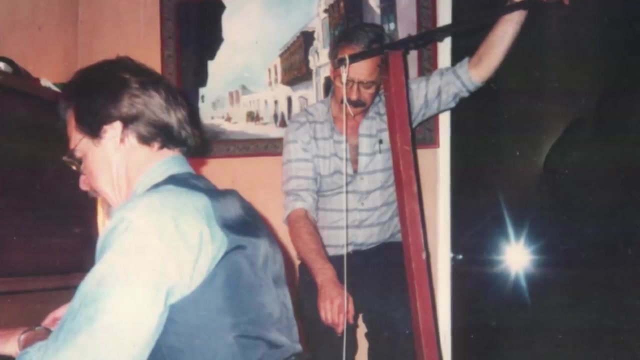 color and a physical feeling. They have four basic terms to describe color, but they're on a spectrum of light versus dark, strength versus weakness and wetness versus dryness. Those kinds of languages don't fit neatly into a color chip identification test. But by the late 1970s,